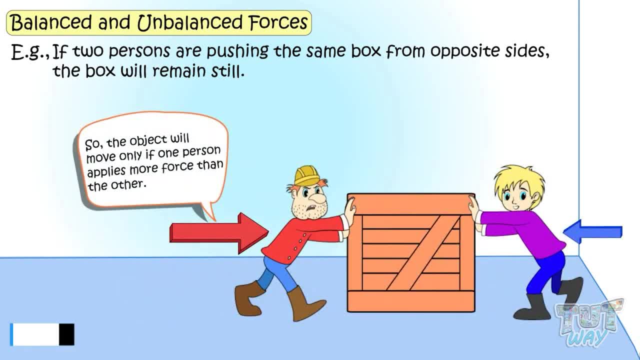 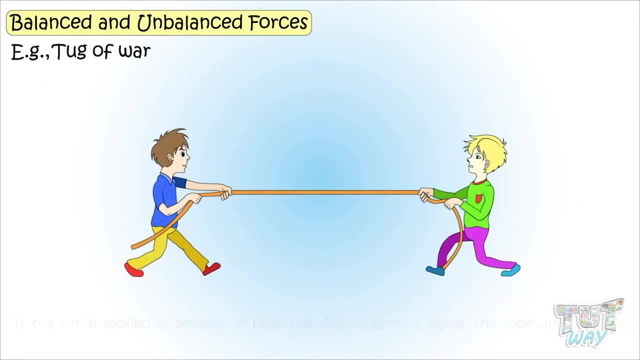 of the persons applies more force than the other, That is, there is an imbalance in the forces. So movement is caused only if unbalanced forces are there. Here is another example: In case of tug of war, if the force applied by persons on both sides is the same or equal, 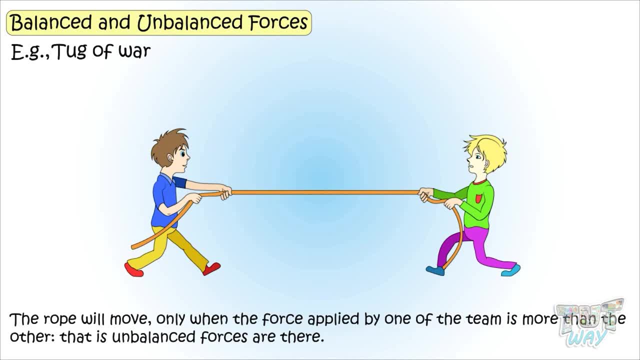 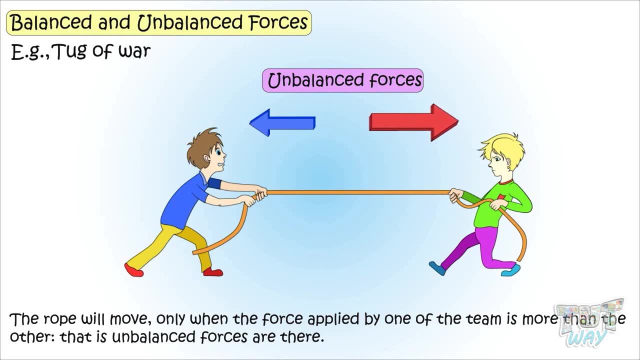 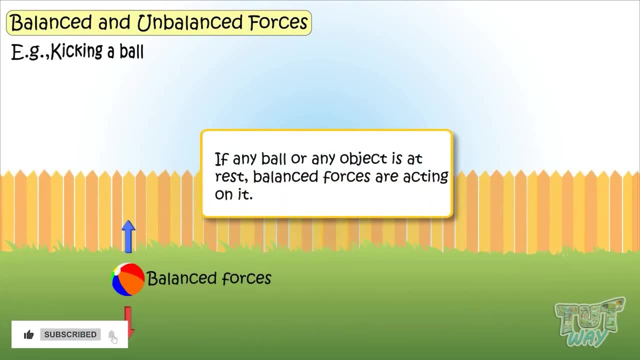 the rope will not move. The rope will move only when the force is applied more by one side of the team than the other. That means unbalanced forces are there. If there is a ball at rest, it means balanced forces acting on it. Then the ball will stay at rest until. 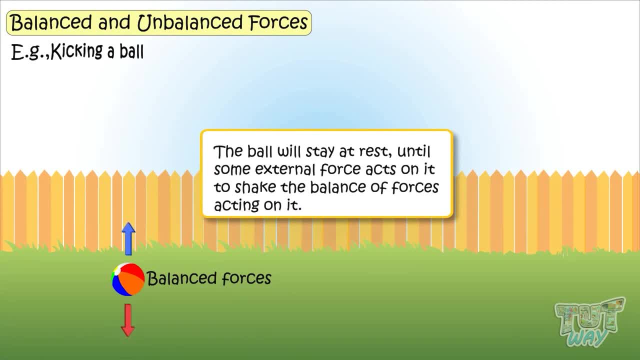 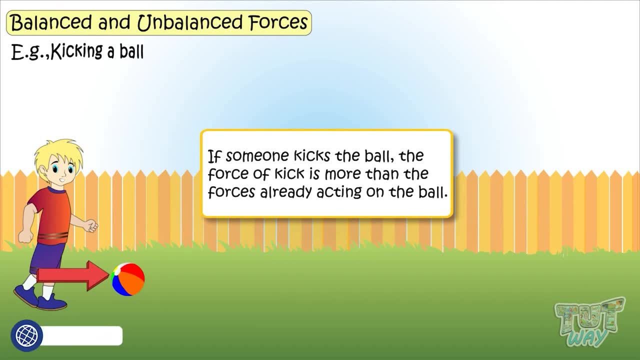 some external forces act on it to shake the balance of forces acting on it. If someone kicks the ball, the force of the kick is more than the force already acting on the ball. That is gravity. is pulling the ball Ground is putting. 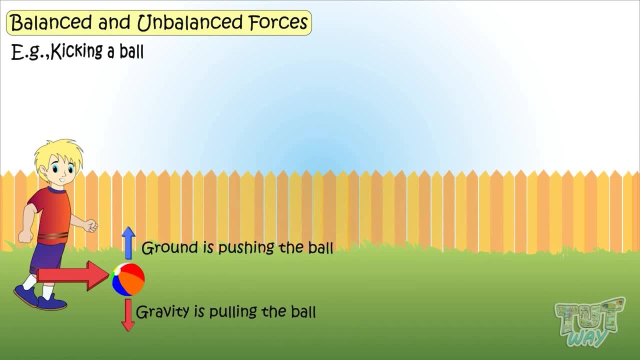 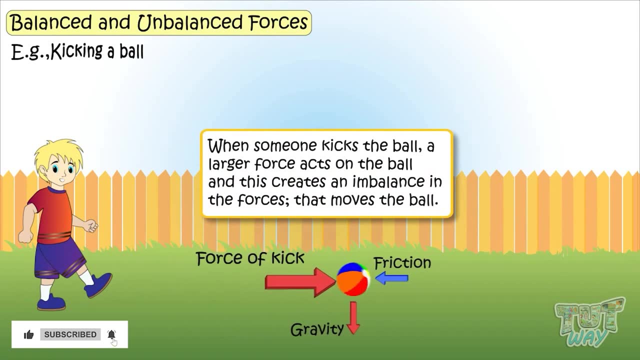 the ball. That is, both the forces were equal and opposite. That is, balanced forces were acting on the ball, But when someone kicks back, it still moves And the flow of the it. a larger force acted on the ball and there created an imbalance in the forces. 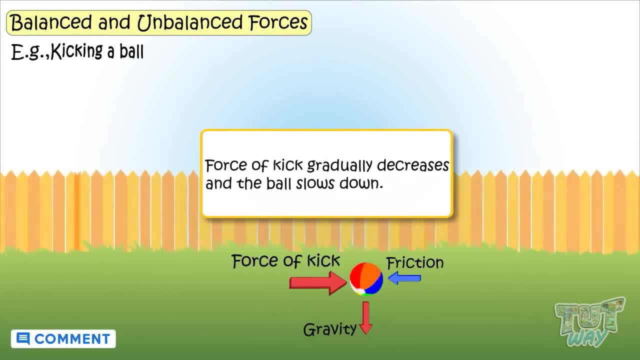 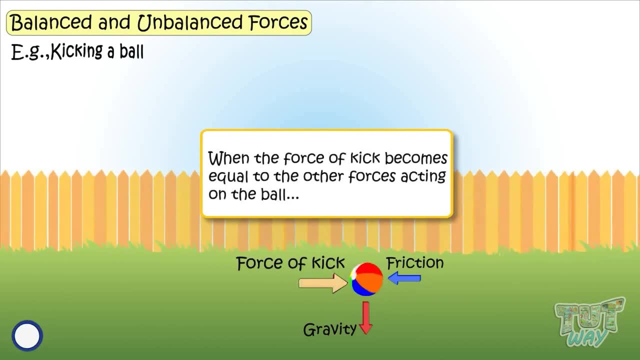 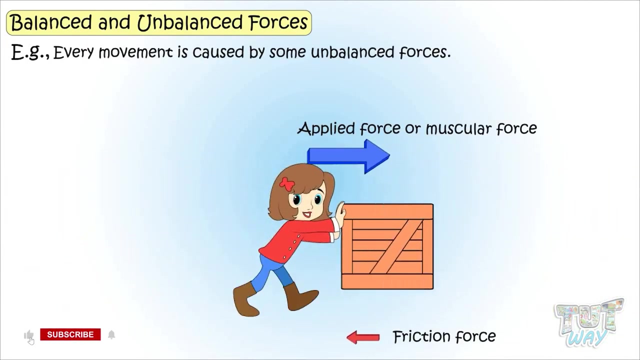 that moves the ball. Now the force of kick gradually decreases and the ball slows down. When the force of the kick becomes equal to the other forces acting on the ball, again balance forces are there acting on the ball and the ball stops. So, kids, any movement is caused by unbalanced forces. When one out of the 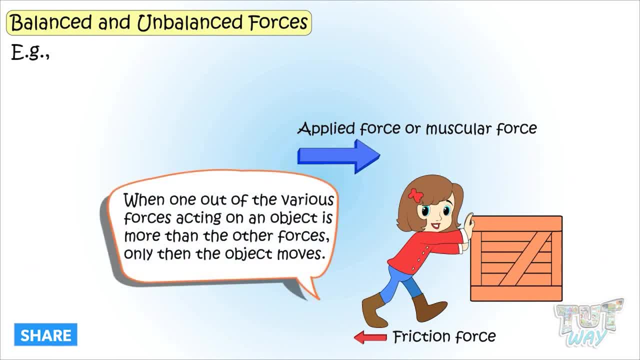 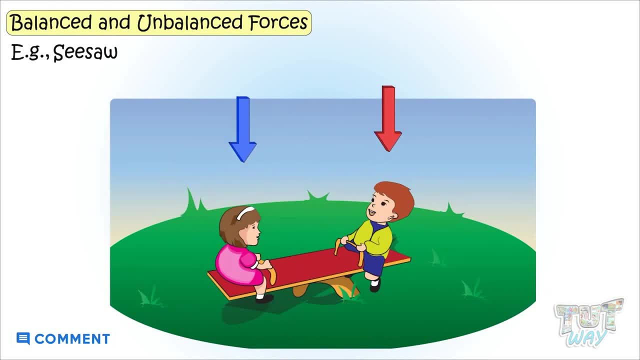 various forces acting on an object is more than others, only then the object moves. Here is an example of a seesaw. It will stay balanced if the weight of both children is the same or the same force is applied at both ends. a heavier person. 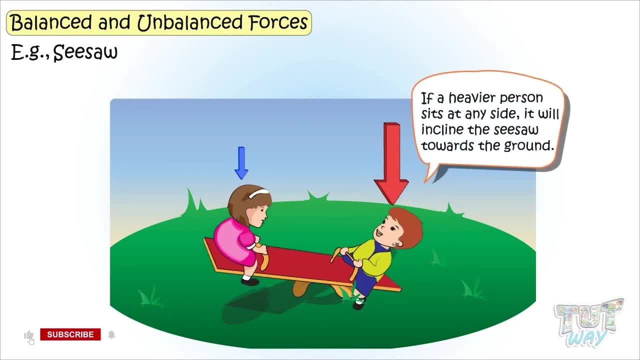 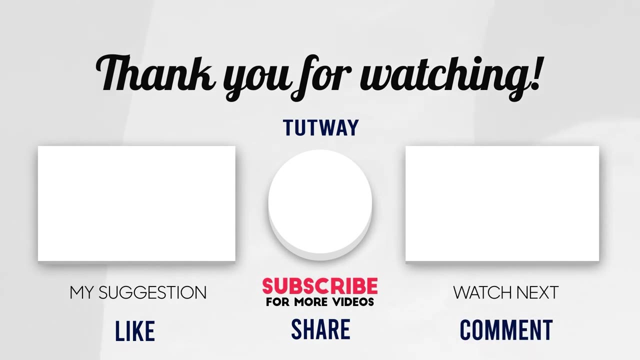 sits at any side, It will incline the seesaw towards the ground. That is, unbalanced forces now applied to the seesaw, So the seesaw moved. Thank you so much for watching. Don't forget to like, comment and share this video, And if you want to see more fun videos, you can hit. 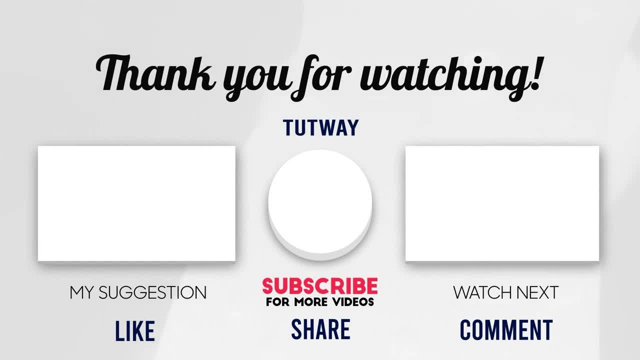 that subscribe button. You can also follow us on Facebook and Instagram for more content. Bye, bye.